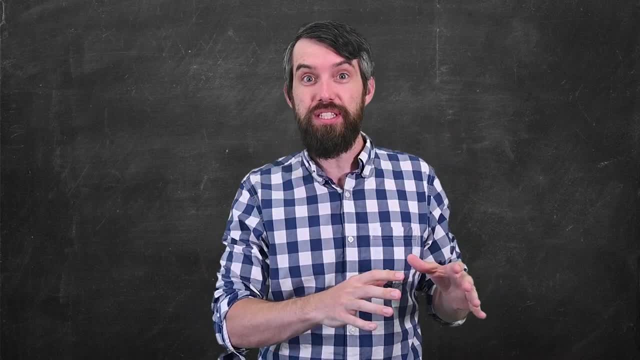 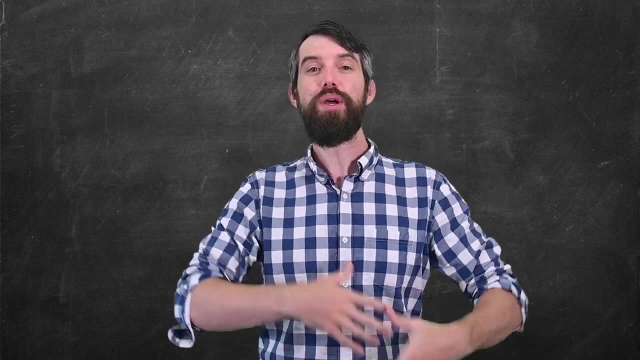 In today's video we're going to investigate the very foundations of mathematics. We're going to take a look at normal mathematical objects like numbers and functions, but we're going to interpret numbers and functions in terms of set theory, in terms of the building blocks of mathematics. 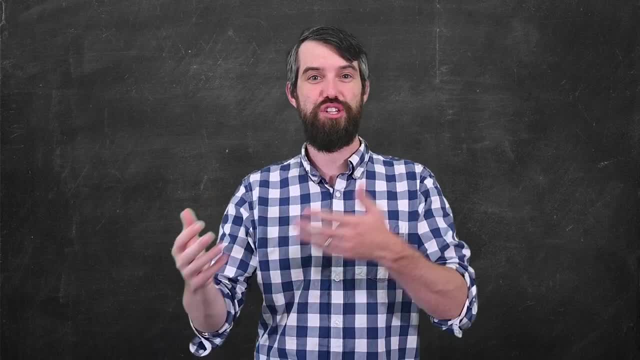 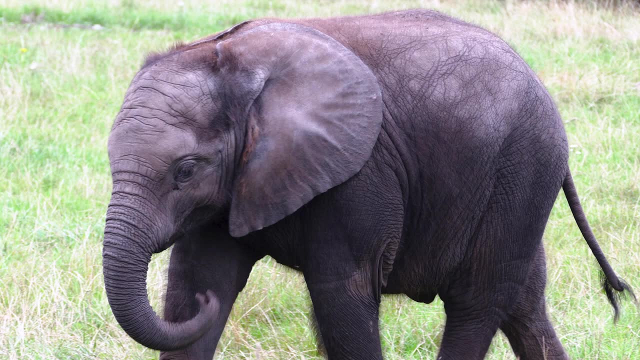 To give you a bit of a feel of what we're doing here, just take a definition of something. It doesn't have to be a mathematical object. How about the definition of an elephant? Well, an elephant is an animal that has a bunch of properties like it's got a trunk and big ears and gray body and so forth. 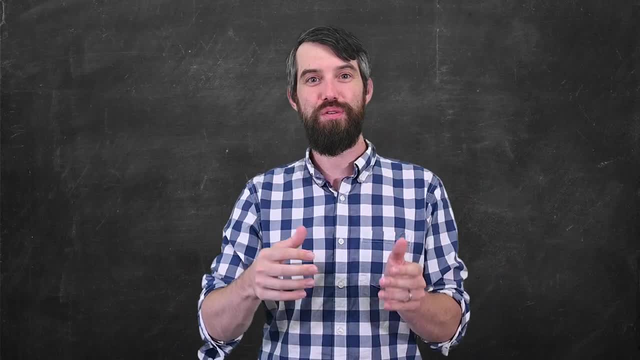 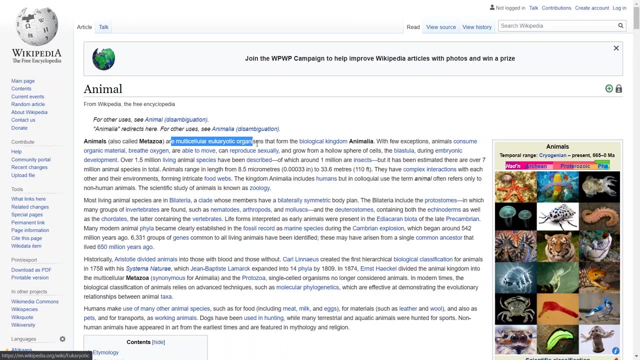 But since the definition of an elephant involves the concept of an animal, we can then say: well, what's an animal? Now, I don't know my biology well enough to answer this, but if I look it up, it's a type of organism. 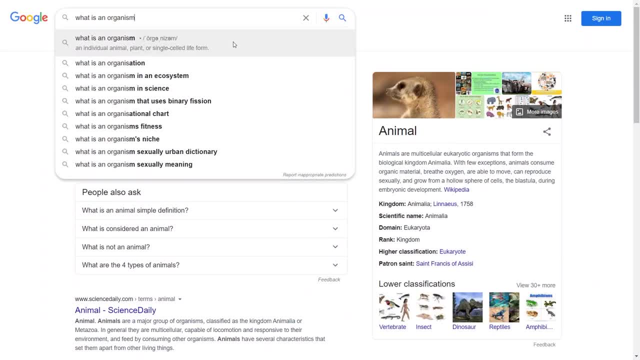 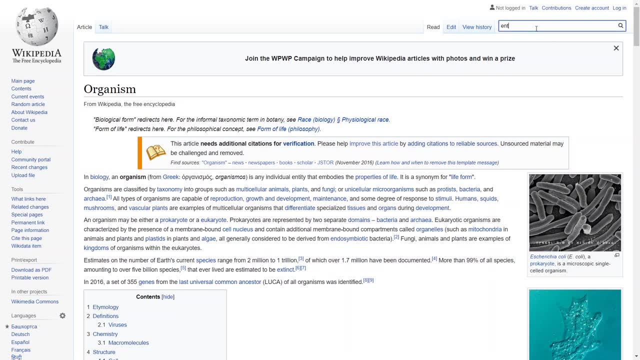 It's an organism with a bunch of different properties. Okay, but then what's an organism? An organism is a special type of entity. Digging further, what's an entity? Well, I'd have to leave Wikipedia here, because there's not an obvious definition of that. 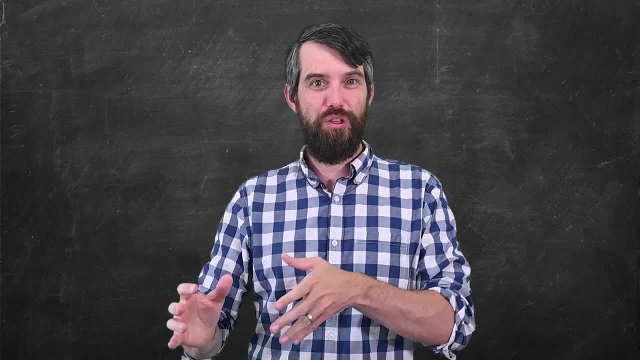 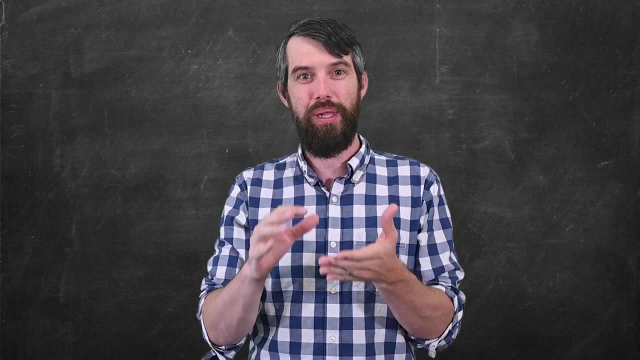 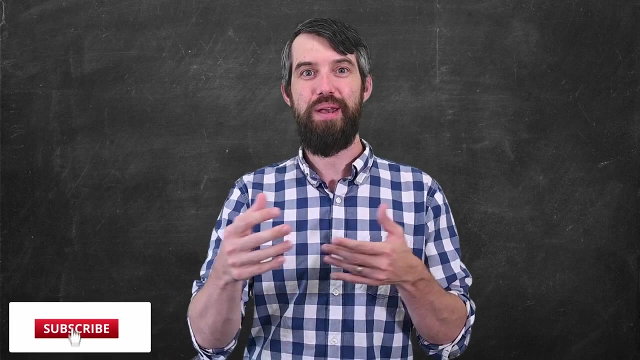 And indeed this is the basic problem. If you take definitions and you keep on investigating the words inside of the definitions, at some point you have to get down to a level where you and I just agree on the foundational concepts. So what does this story look like in mathematics? 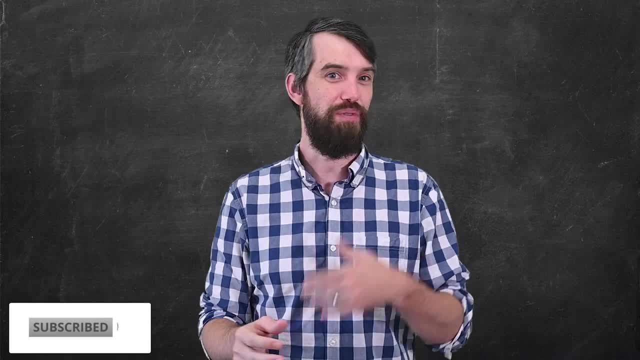 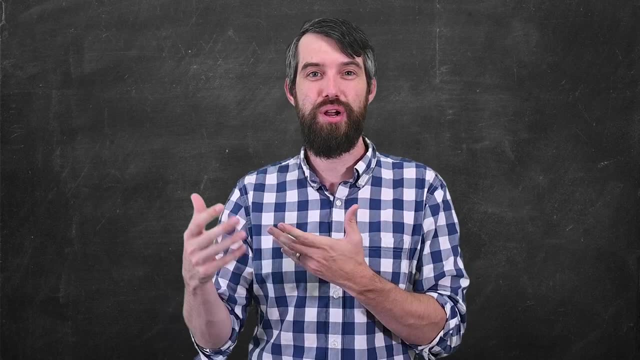 If you take some definition of a concept in mathematics, we've got numbers, we've got functions, vectors, matrices. As you go on, in mathematics there's going to be increasingly esoteric concepts, fields and categories, and manifolds and any number of other things. 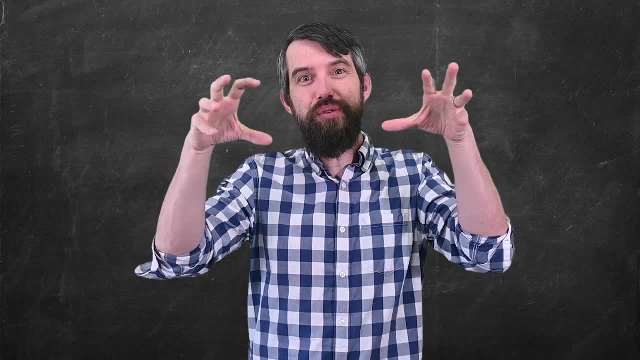 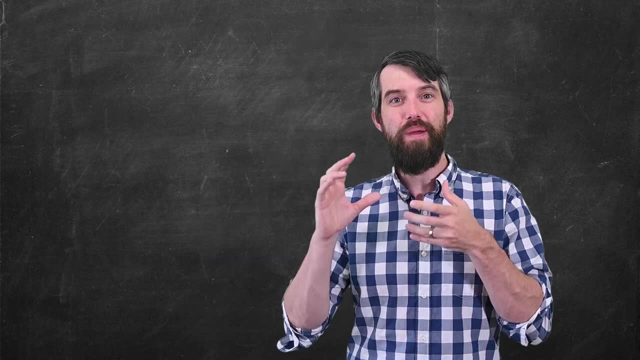 But if you look at all of the words and all of those objects, what do they reduce down? if you keep investigating what the definitions of mathematical words are Now, it turns out that one of the major ways to do this is to ground everything in set theory. 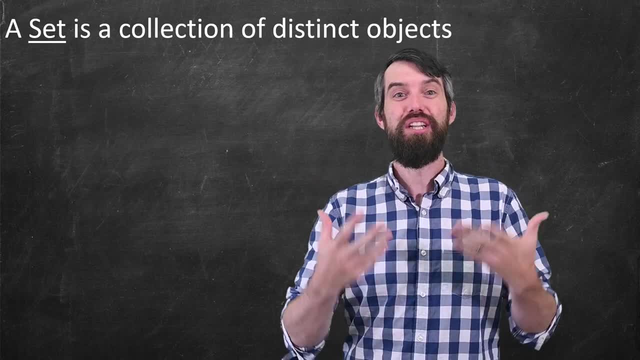 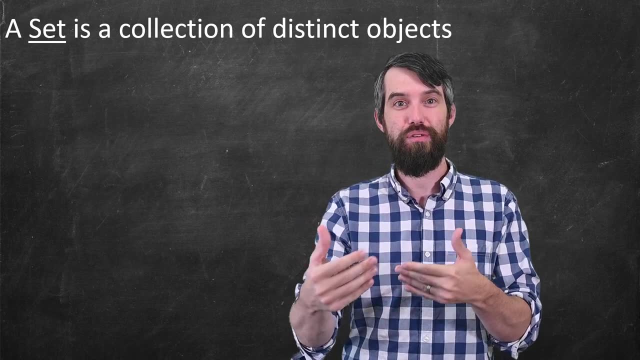 So this is the definition of a set. A set is a collection of distinct objects. Now I'm just going to say that you and I have to understand and agree on the notion of what this set is. These words that I'm using are just descriptors for you and I to try to understand it. 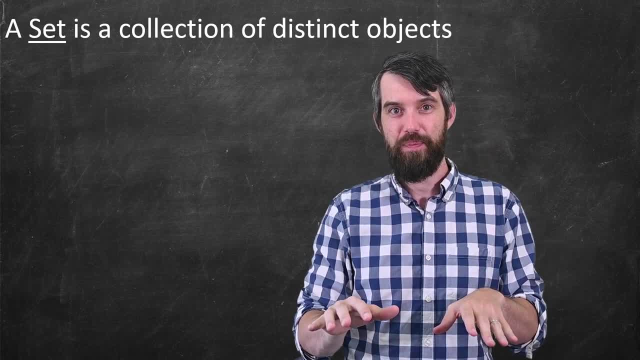 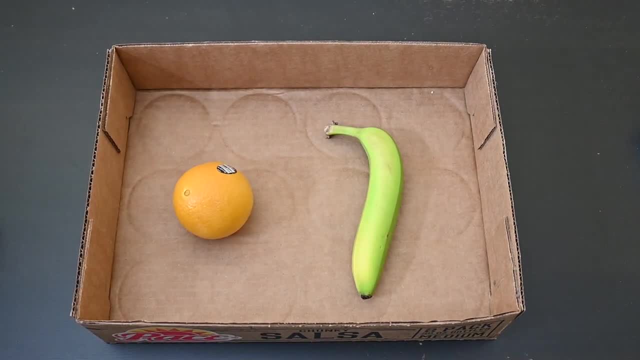 But I'm not going to go any further than this. This is my base. The way I interpret this is a set is just a box with different types of things in it. For example, this is a set that contains different types of fruit: a banana and an apple. 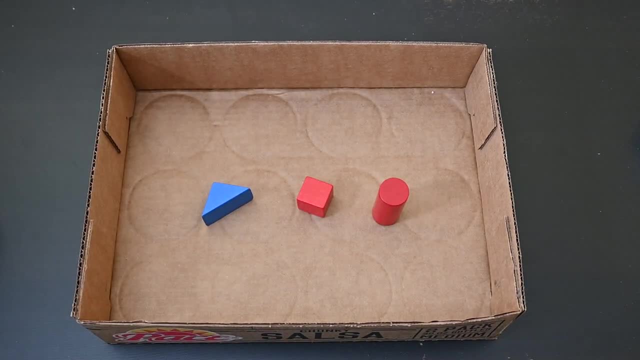 And that this is now a set that contains different types of blocks. The individual objects inside of this box, inside of this set, refer to as elements, So this is a set with three different elements. The fact that I say they have to be distinct objects basically means I just can't put the same object in twice. 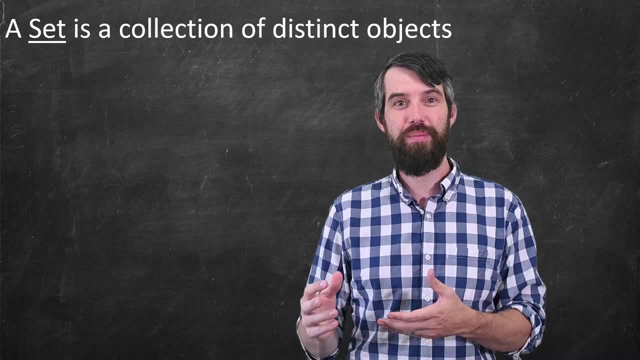 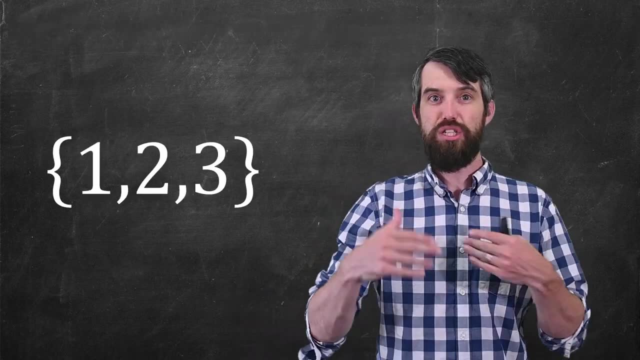 I sort of think about it like a sports team. A sports team can have one player on the team. You can repeat their name 300 times, but there's still only one player that's going to be on that particular team. Let's look at some mathematical examples of sets. 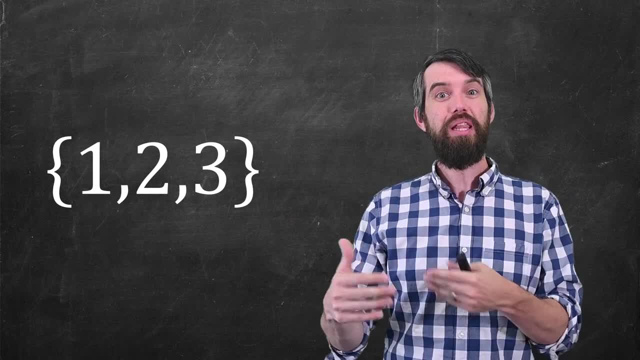 So, for example, this is the set 1,, 2, 3.. The squiggly braces here are sort of like a set. They're sort of like the box that we saw before. They say I'm talking about a set of objects. 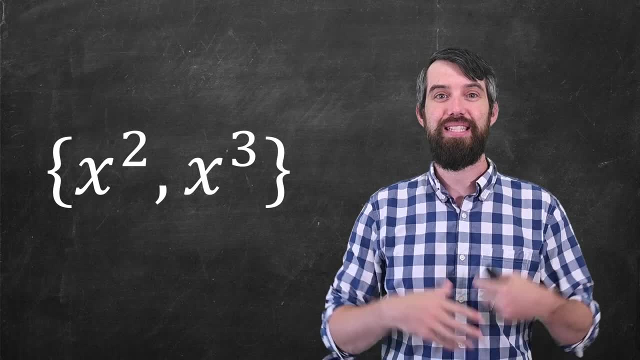 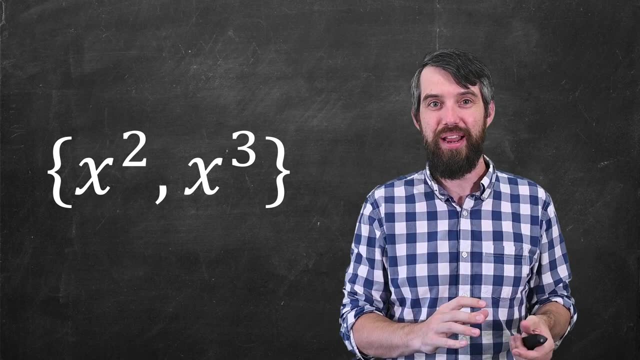 In this case I'm talking about the objects 1,, 2, and 3.. This is a different set. It is a set that contains functions: The function x squared and the function x cubed. And then there's one very special example of a set I'm going to illustrate. 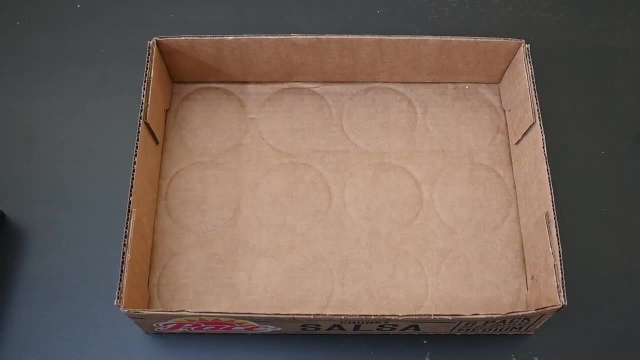 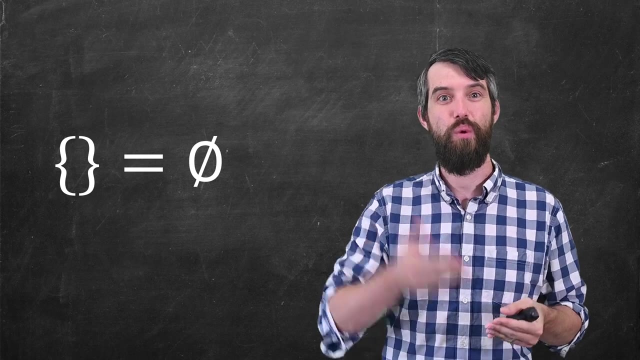 It's the set with nothing in it, Squiggly brackets with nothing. This is an empty box And we give a special symbol to associate to that set. We sort of zero with a backslash to it. This is the empty set. 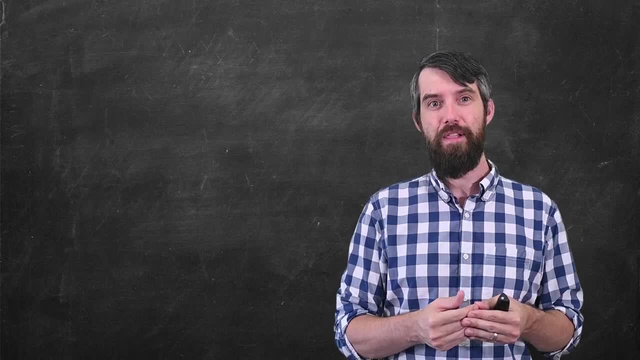 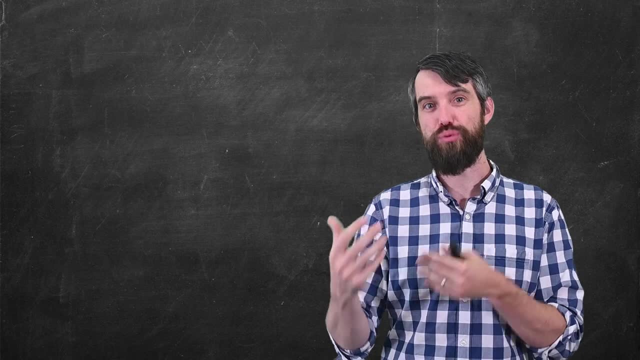 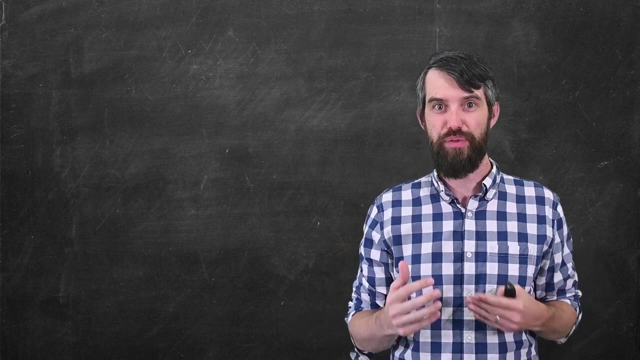 Note that mathematicians do actually go a bit further than just agreeing, as this is a foundational concept. There's a list of axioms that specify the different properties that sets have to have. The Zermelo-Fraenkel axioms are the most standard way that mathematicians have agreed on the basic concept. 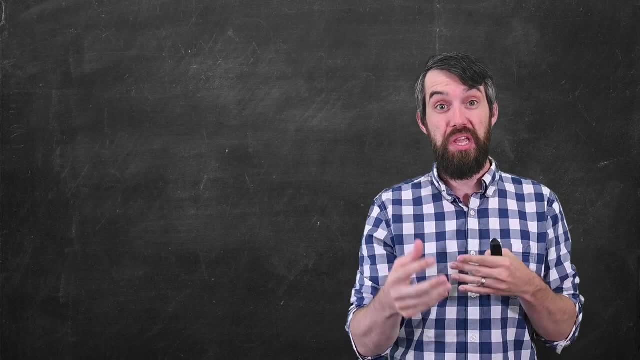 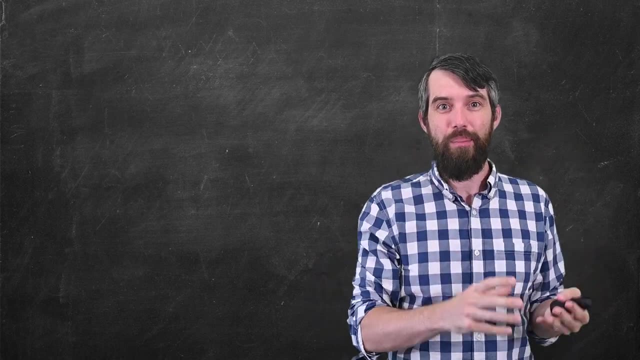 But either way, we're saying: this is the base and we're all just going to agree on what that means. Okay, so let's do something with that. I want to now interpret what is a number, Because a number is not a set. 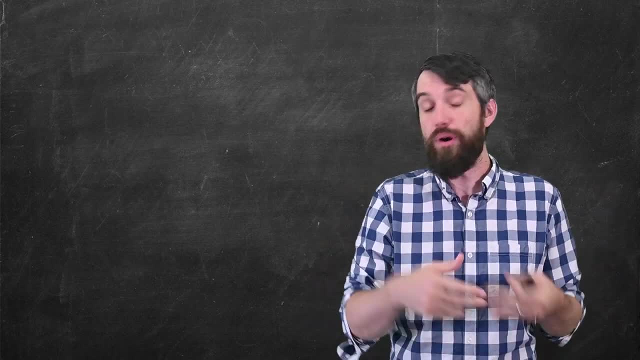 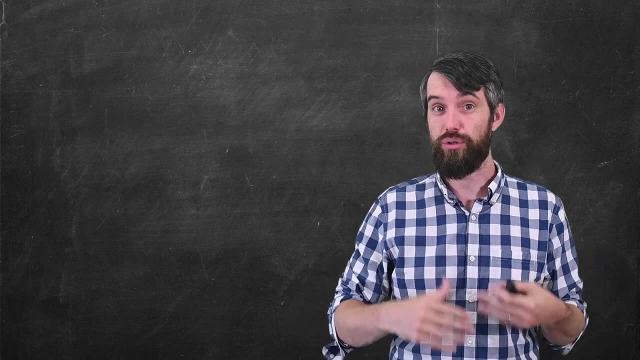 I've talked about the set that contains numbers, but what really is a number? Could I interpret numbers as just being a special type of set? So basically, what I'm going to do is I'm going to look at the natural numbers 0,, 1,, 2,, 3, and so forth. 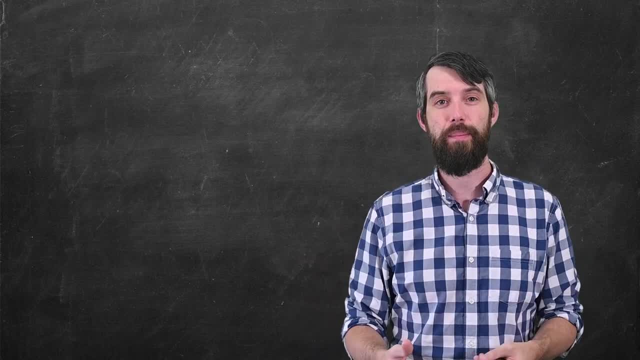 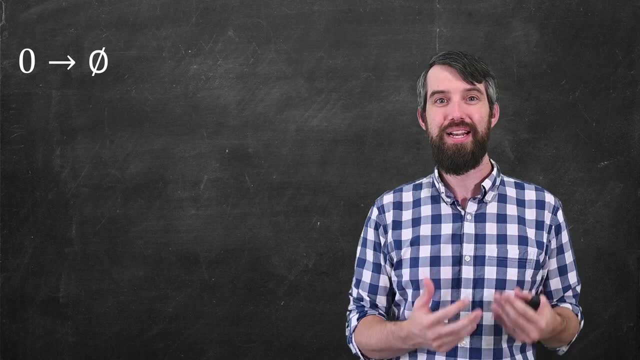 and try to associate a particular set to each of them. So the first one I'm going to do is I'm going to associate 0 with the empty set. I've drawn an arrow here relatively loosely, And what I'm trying to say is that the concept that you and I have in our minds of 0,. 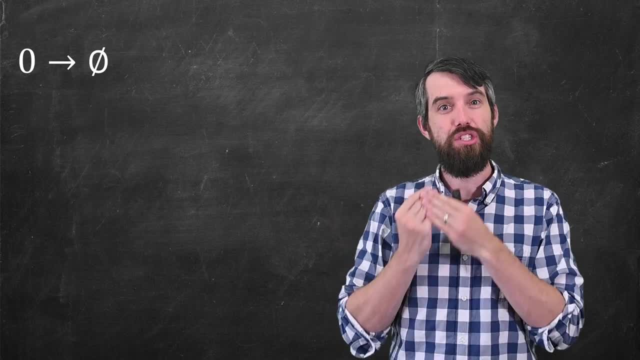 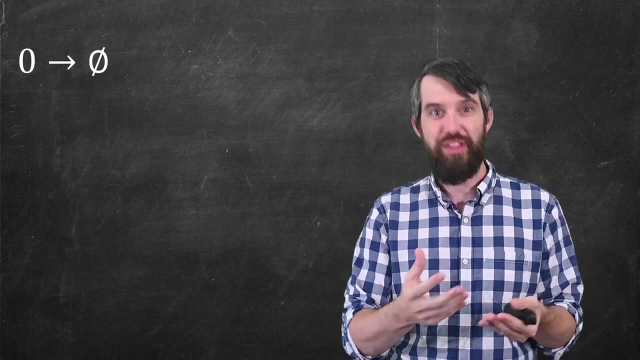 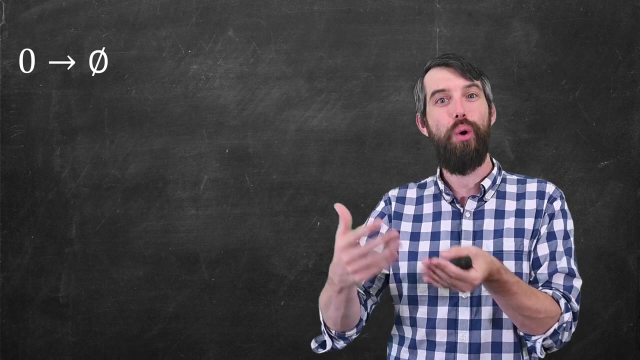 I'm going to interpret that in terms of the language of set theory, by associating to it the empty set. Indeed, the empty set is not nothing, It is a set with nothing inside of it, And so this association makes sort of sense, because I'm associating 0 with the set that has 0 elements inside of it. 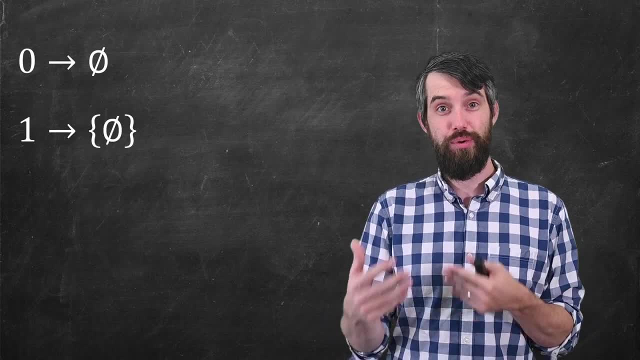 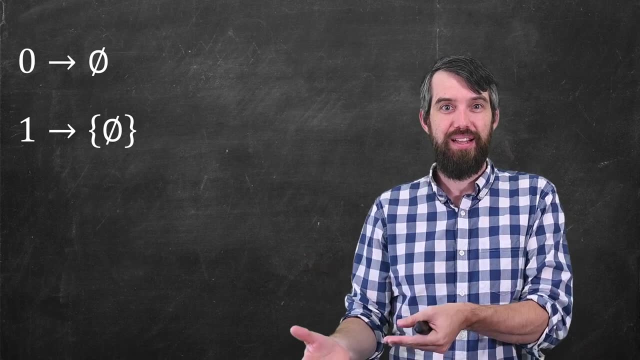 Likewise, let me take the number 1.. And 1 is associated to a set as well. It's associated to the set with one element in it. The element is just the empty set. So I think of this as a box. that's the big outside set that contains the empty set. 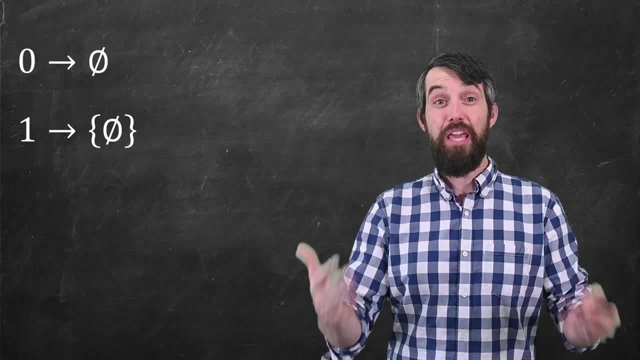 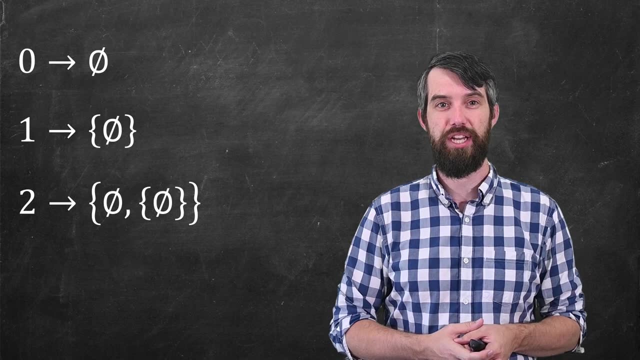 This is a box within a box. Okay, let me keep going. What about 2?? 2 are defined to be a special type of set that has two different elements into it, So let's make this different. association 2 is the set that contains, well, both of the previous ones. 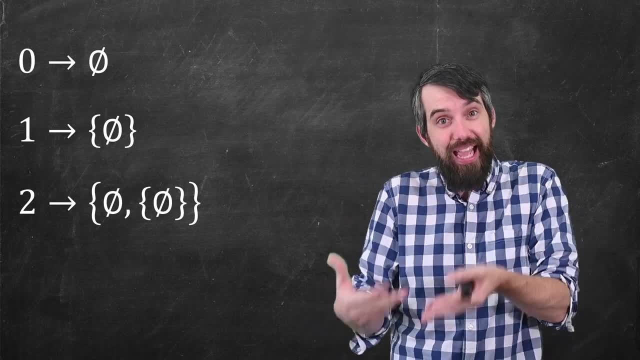 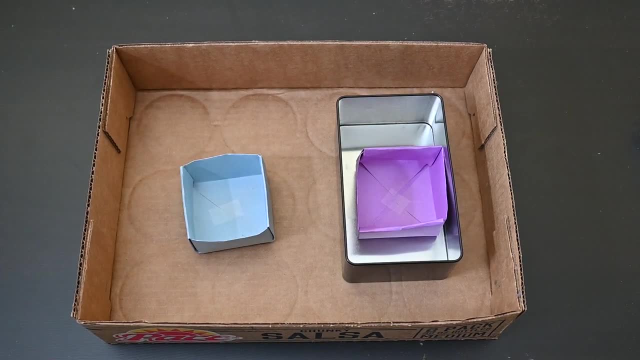 It contains the empty set And it contains the set that contains the empty set. So, in other words, at the level of the outside box, this biggest box, there's two things inside of it: There's an empty set, an empty box. 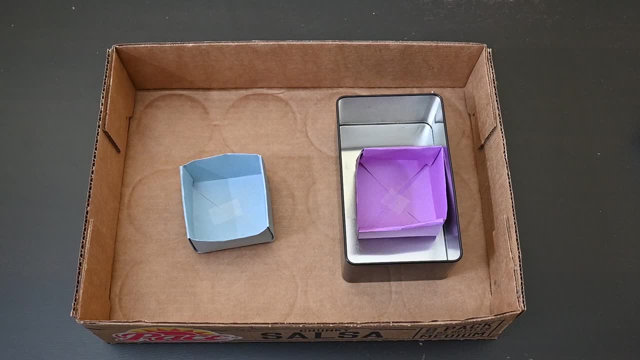 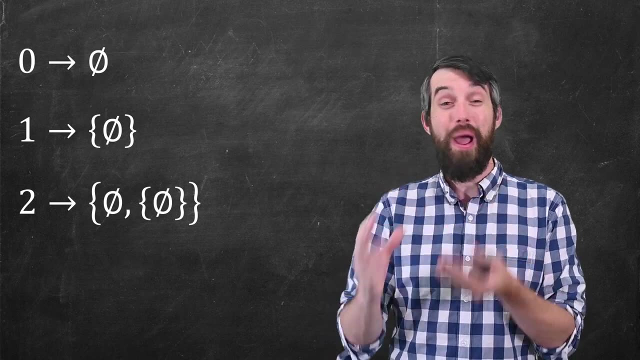 And then there's a box that contains an empty box, There is the set that contains the empty set. Okay, so, continuing with that pattern, let's try and see how I can write a number 3 in a way that sort of makes sense. 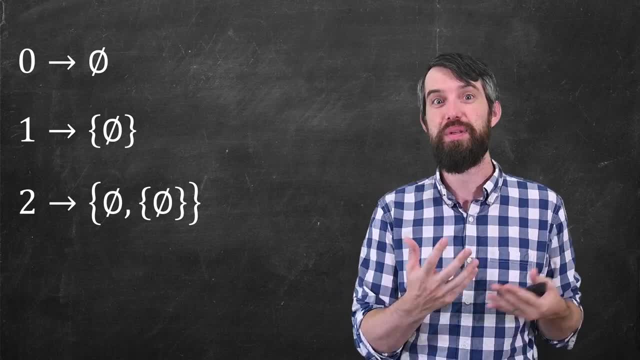 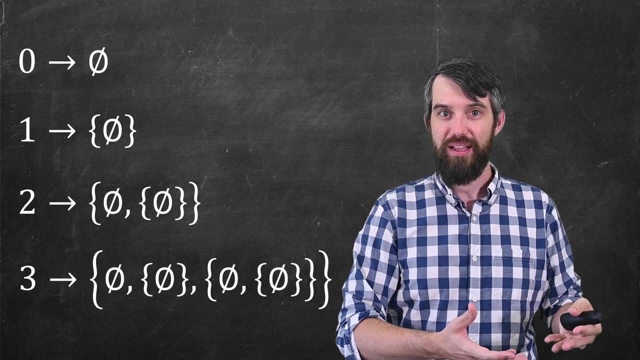 and label it as the symbol that we'll use as a shorthand for a particular type of set. I can do the same thing. I want a set with three elements in it, So in this case I'm going to have the set which has got the empty set. 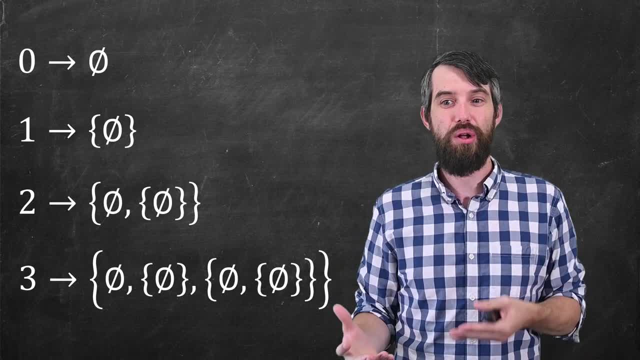 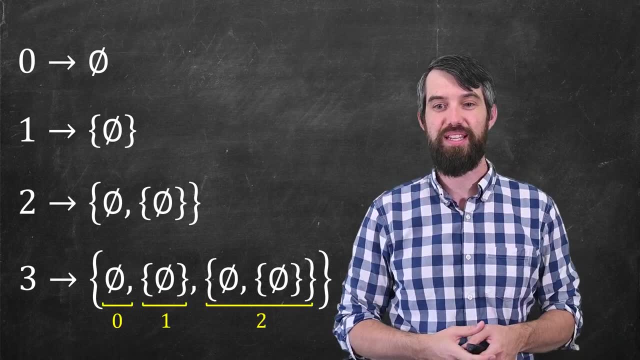 the set that contains the empty set and the thing we previously called 2, the set that contains the empty set and the set that contains the empty set. It's much shorter to just treat it as this: is the set that's containing 0,, 1, and 2.. 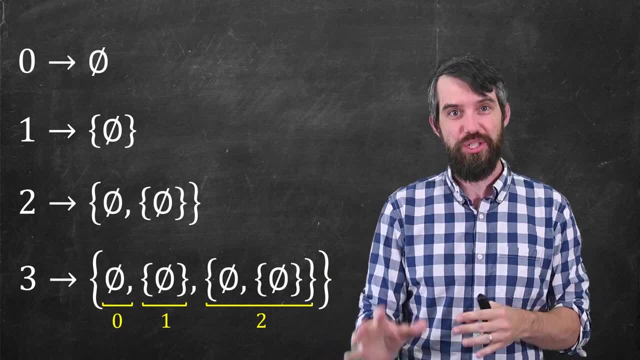 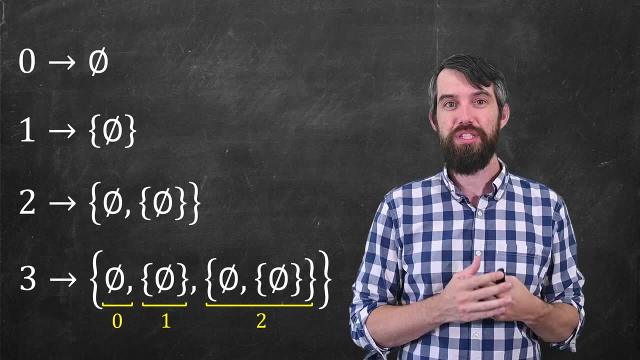 Now this might seem very weird and bizarre, and that's correct. It is a bit strange. We would never normally prefer to write numbers in this way. The advantage of doing this is recognizing that numbers can be thought of as nothing but sets. 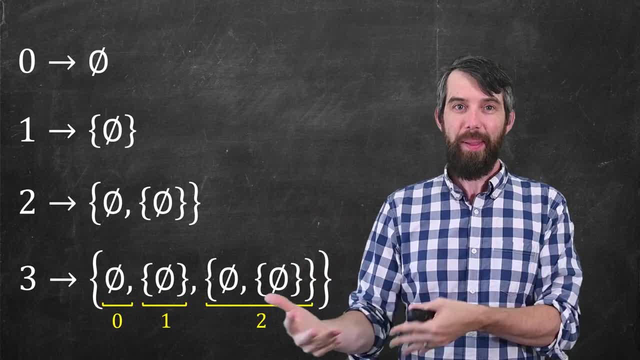 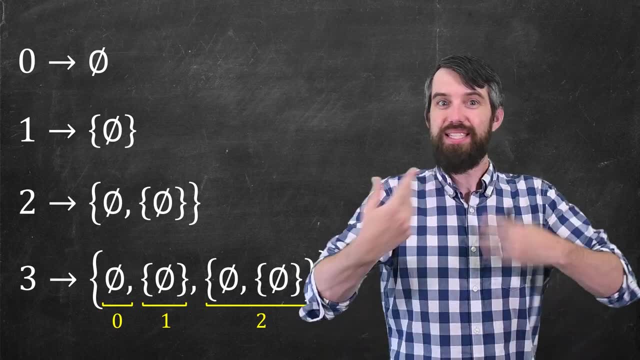 We've agreed on the concept of a set and now more complicated things like the number 3 is just a particular type of set And there's nothing in here except for sets. There's sets, There's sets. inside of sets. There's empty sets. 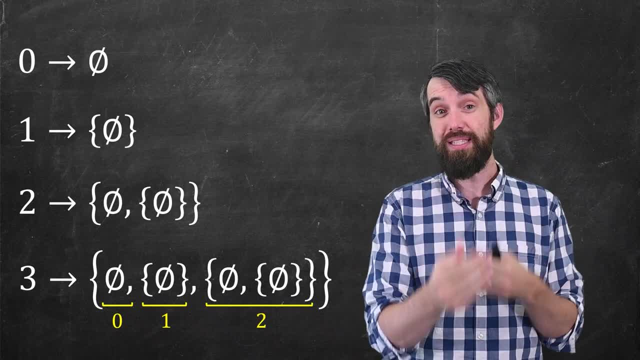 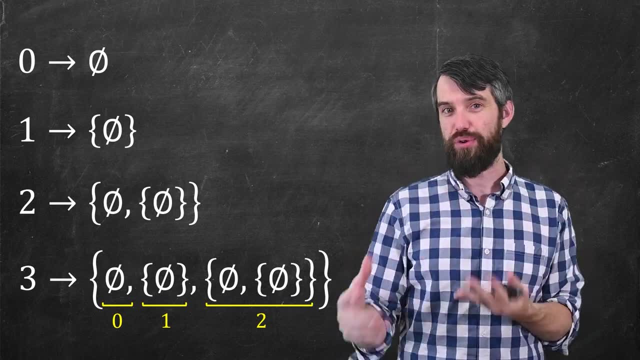 But it's just sets. So if you and I accept the concept of a set now, we have to understand that we accept the concept of 3 when I write it in this particular way, And similarly I could write all natural numbers in this way. 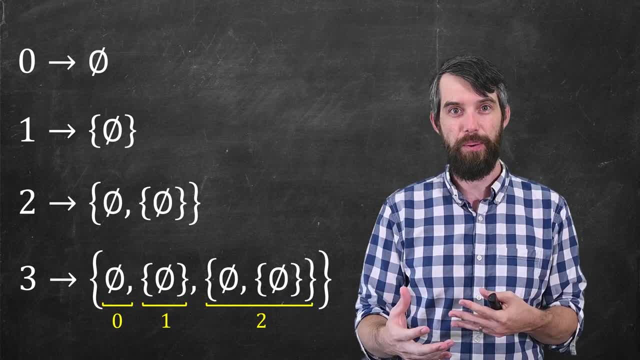 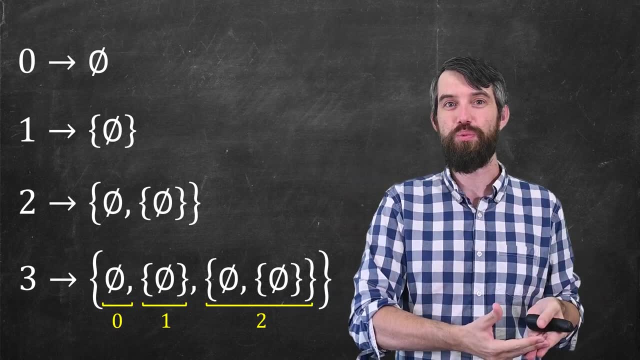 We just get increasingly complicated, but the pattern, I think, is clear. So now, if you believe in the concept of sets, you can believe in the concept of numbers as well, because we've written numbers in terms of sets. But what about something more complicated? 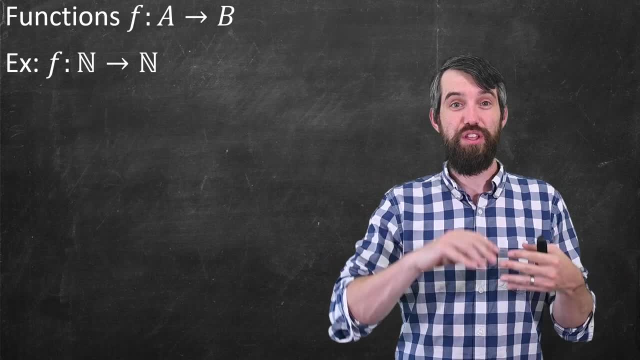 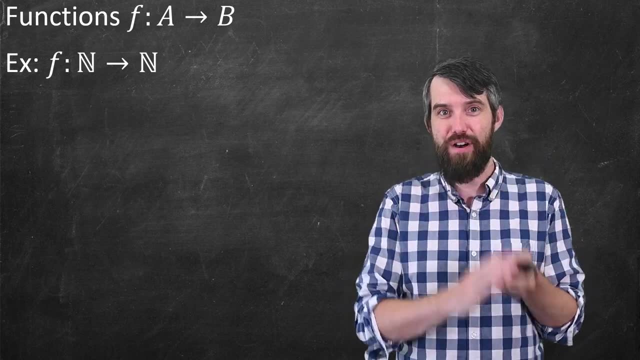 What about functions? Imagine I've got a function f that goes from a to b. We've seen examples of this, like, I don't know, the function x squared, So maybe I'll use that as an example. I'm going to actually take a function from the natural numbers to the natural numbers. 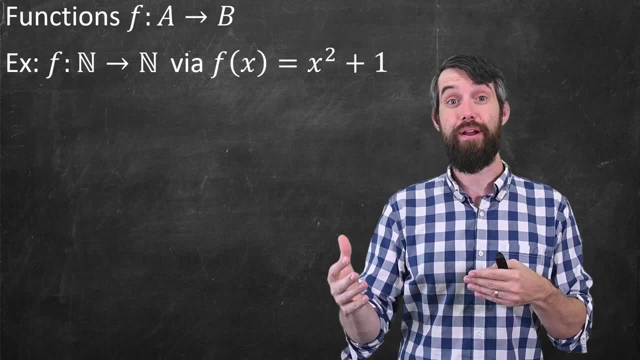 so numbers like 0,, 1,, 2.. And the function I'm going to take is the function x squared. Actually, I'm going to do x squared plus 1.. Functions are much more complicated than numbers. Numbers are just sort of a set. 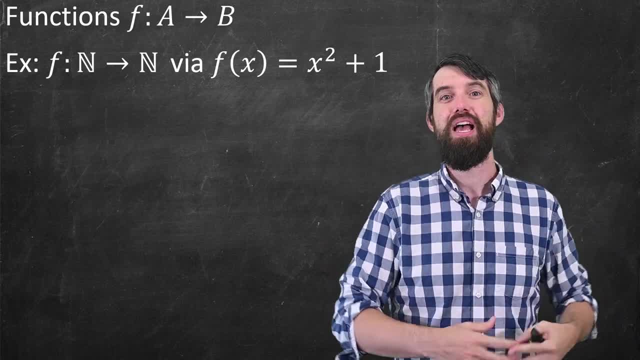 They just sit there. But functions have an input, a domain That's the set a. They have an output. A codomain is sometimes called the set b. They're sort of dynamic. They take things from the one set to the other set. 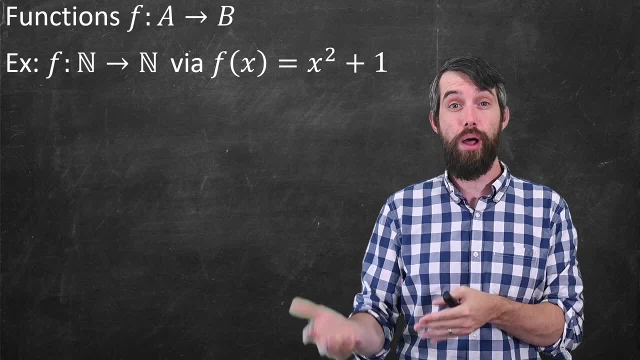 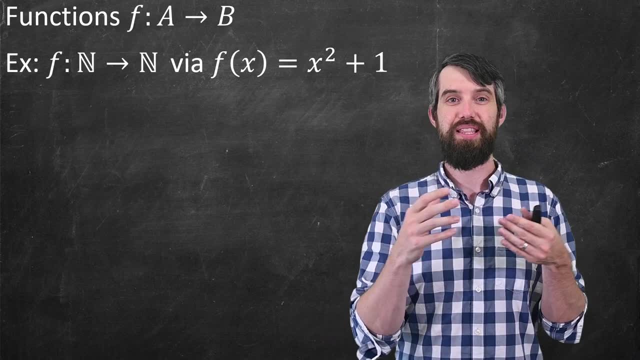 Functions are a much more complicated mathematical object, So do we need a new base, or is set theory enough for that? Well, indeed, it's going to be enough. Now, what I think of when I take this function, x squared plus 1, is I can just plug in different input values. 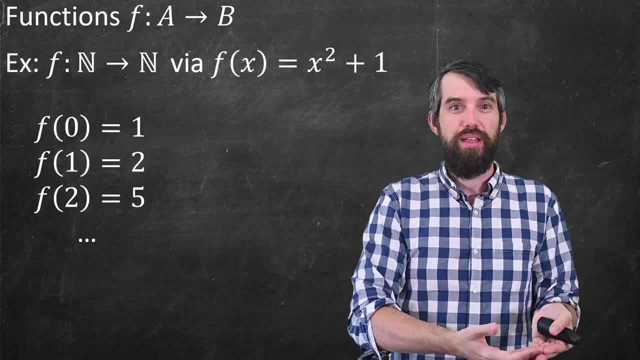 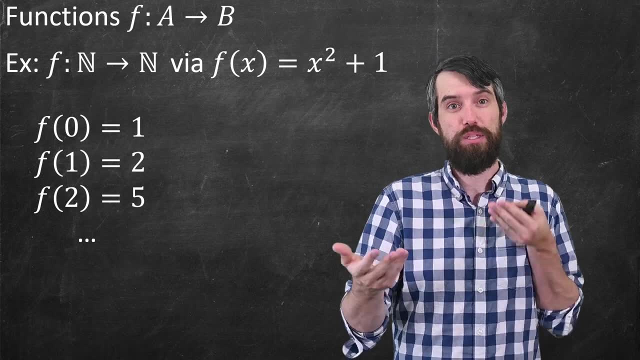 So, for example, the function at 0 is 0 squared plus 1, which is 1.. The function at 1 is 1 squared plus 1, which is 2.. And the function at 2 is 2 squared which is 4 plus 1, which is 5.. 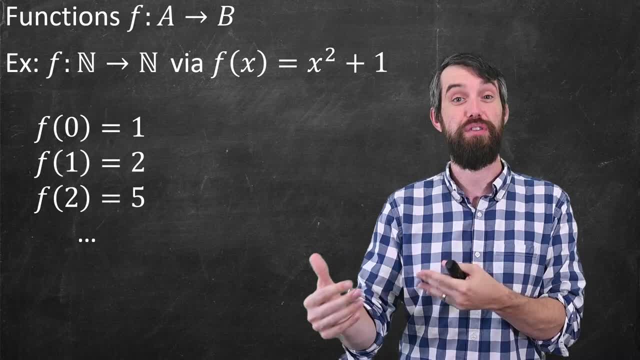 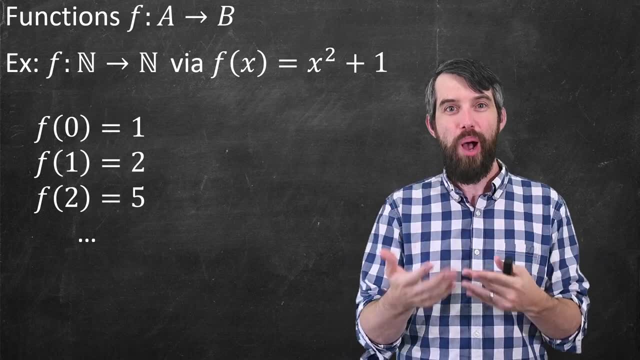 So I've just plugged in the value of this function a few different times. So here's my challenge to you: Can you pause the video and try to come up with some way to encode this information, to encode this concept of a function using just sets? 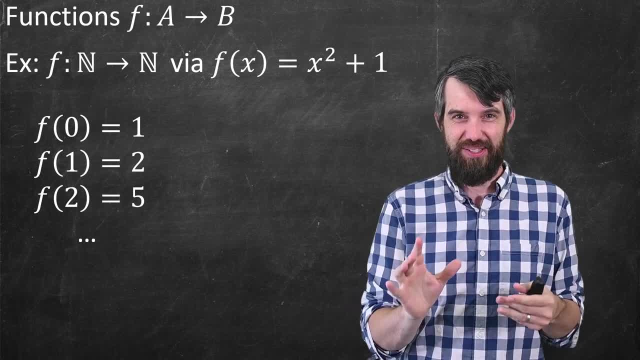 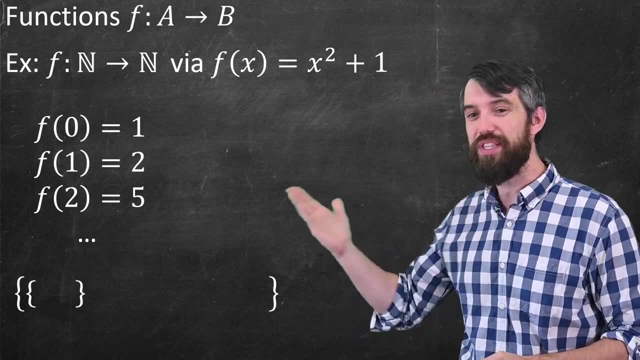 So take pause on the video and see whether you can do it. OK. so let's see whether you guessed the first thing that I did. That turns out actually not to be a good answer. My first guess was this: It's a set. 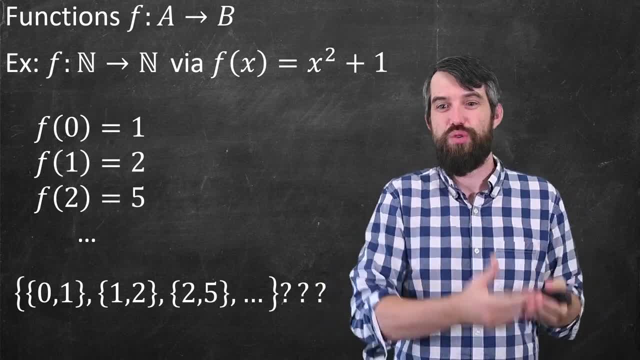 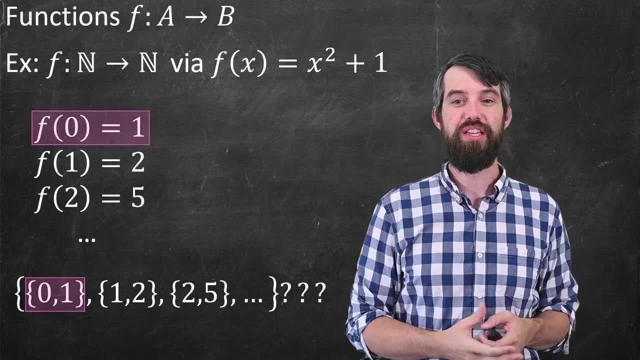 It's a set that contains a lot of other sets like 0, 1, 1, 2, 2, 5, and so on. The reason I thought about this was that there's sort of an obvious encoding f of 0 equal to 1 is encoded by the set that contains 0 and 1.. 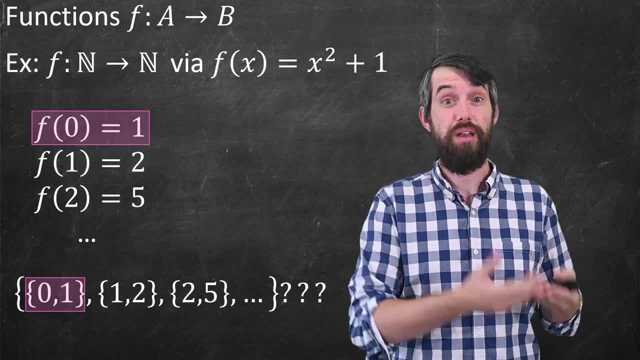 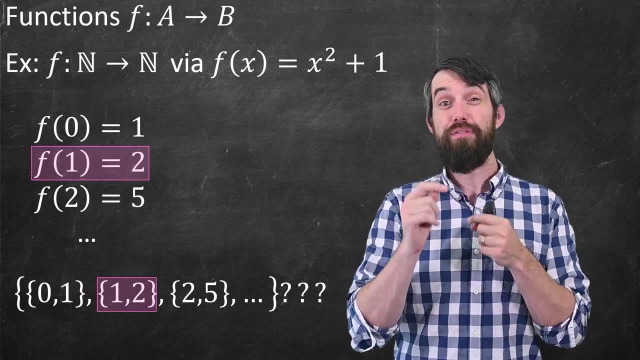 And if we understand 0 and 1, which I argued previously that we do- then we can understand that concept. Likewise, f of 1 is equal to 2 would be encoded by the set that contains 1 and 2.. And the issue here is something we haven't talked about yet. 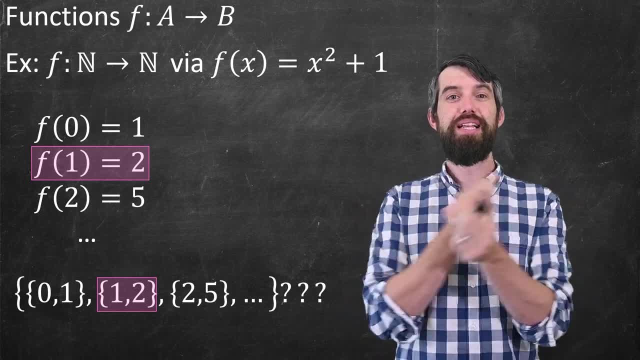 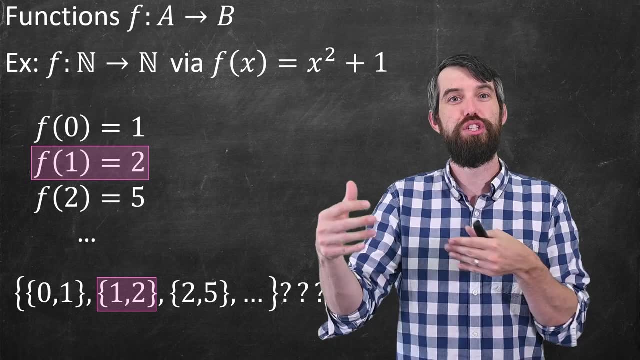 in terms of our concept of a set. A set is something where the order doesn't matter. My intuition here is that it's like a box or like a sports team. It doesn't matter how you move the objects around in that box. It doesn't matter which you list first or second. 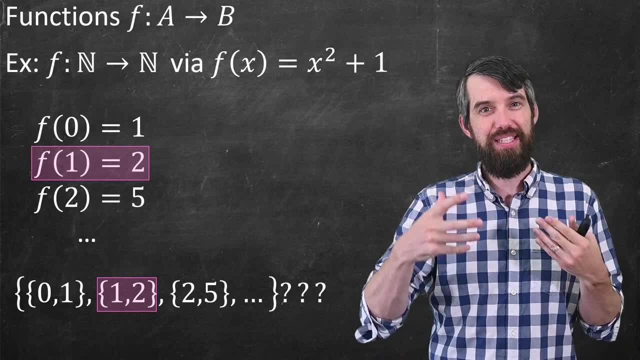 So, in other words, the set 1, 2 and the set 2, 1 are thought of as exactly the same thing. It's just a box where there's a 1 in it and there's also a 2 in it. 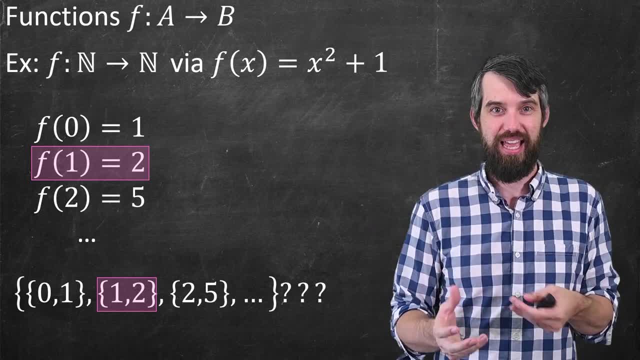 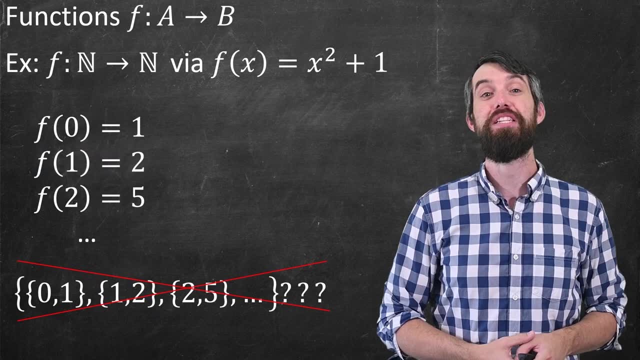 The order doesn't really matter, And so I can't tell by putting this thing, this set with 1 and 2 in it, whether I'm saying f of 1 is 2 or f of 2 is 1.. Unfortunately it doesn't quite work. 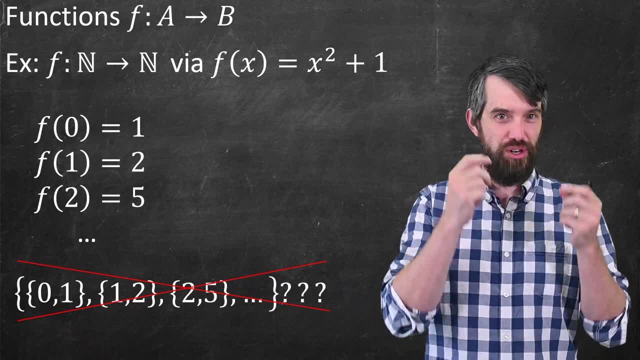 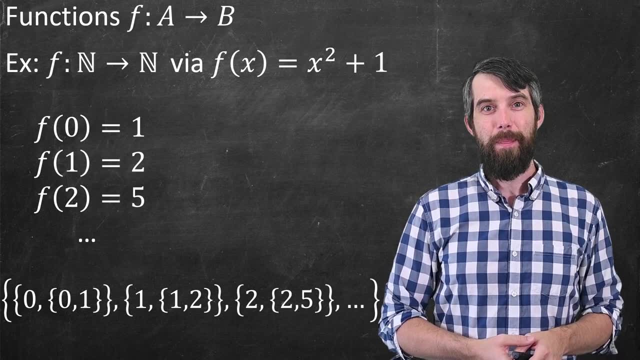 So here's a slightly better method that makes it clear that sort of tags: what is the input and then what is the output. It's going to be a bit long and messy, so let me just write it down. Well, the idea is I want to encode first that f of 0 is equal to 1,. 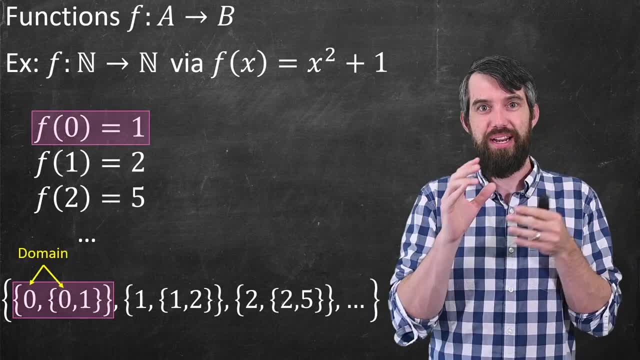 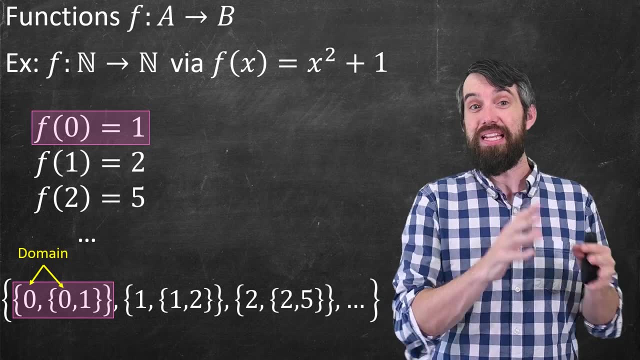 and I do that with this first expression. The 0 here is occurring now in two different places. The 0 first occurs by itself, And the way we interpret this is that if I leave it by itself, just a 0 there, then I'm saying: 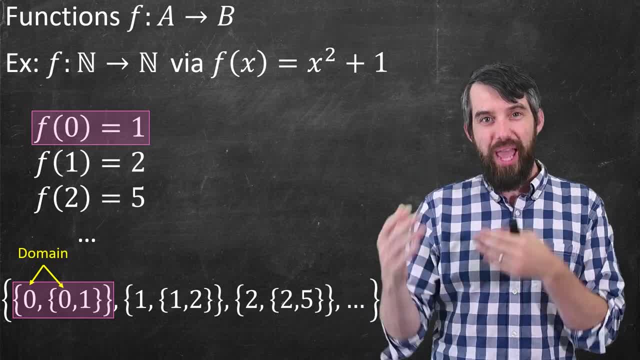 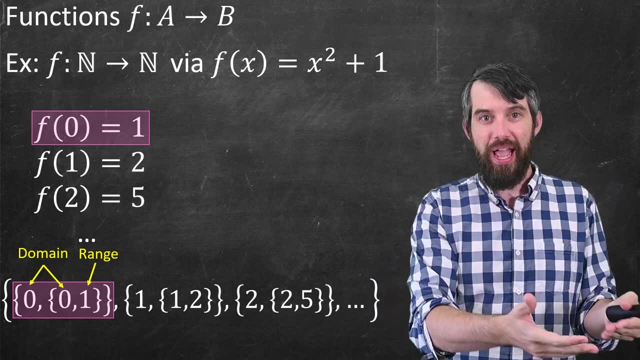 that is the thing that is in the domain, And then I'm pairing that with a 0, 1, like I had previously, And then the 1 here is the element inside of the range. This is where 0 is sent. So when I look at this entire thing highlighted in the pink here, 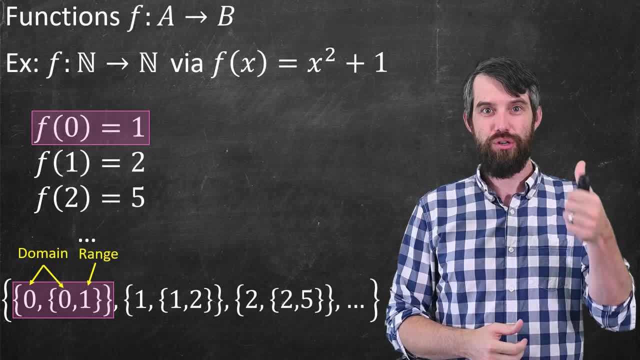 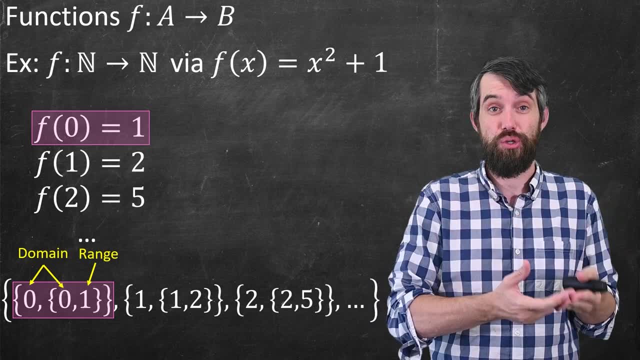 it basically is a way for me to read off that 0 is the 1 by itself and so it's the thing in the domain. And then if I want to know where 0 goes, I look at the brackets- 0,, 1, and it says: 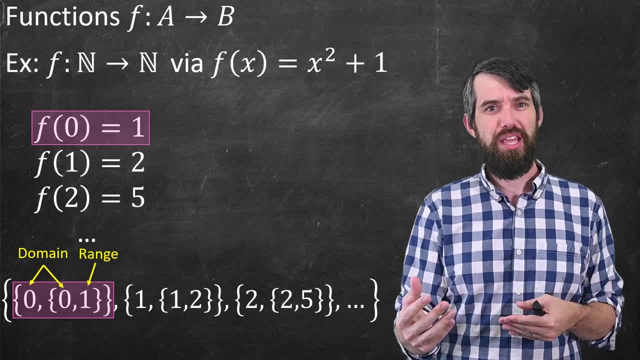 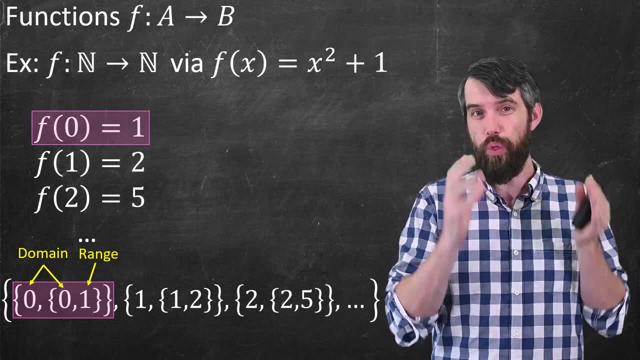 okay, 0 is sent now to 1.. And then the ambiguity of whether I could change the order and write it different ways is gone now, because I told you what the thing in the domain is: It has to be 0. That's the 1 that I wrote by itself. 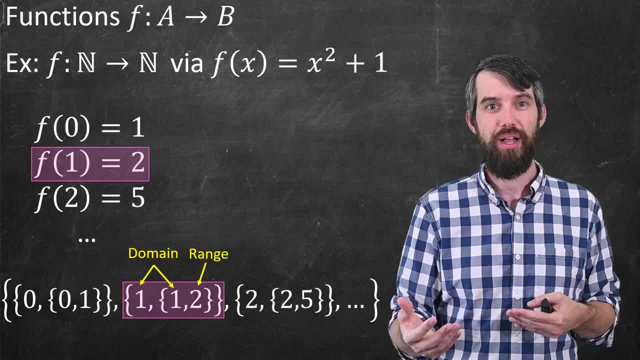 Likewise, if I go along here I can look at the 1 where f of 1 is going to 2. So I put 1 out by itself And then I go and put in squiggly braces the 1,, 2,. 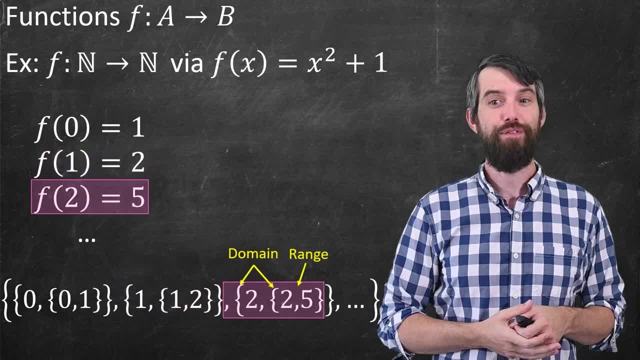 and that just tells me that the 1 is going to be sent to 2.. Likewise the 2,, 5, 1, I put the 2 out by itself. It tells you 2 is the 1 in the domain. 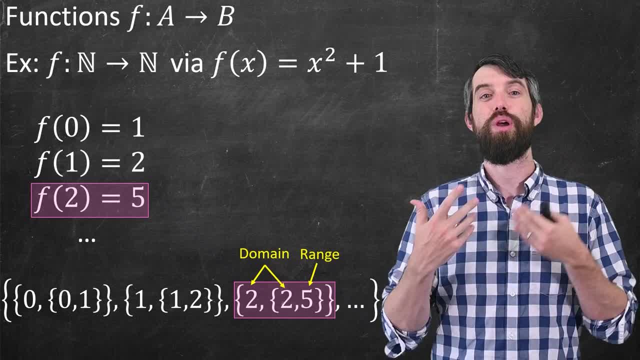 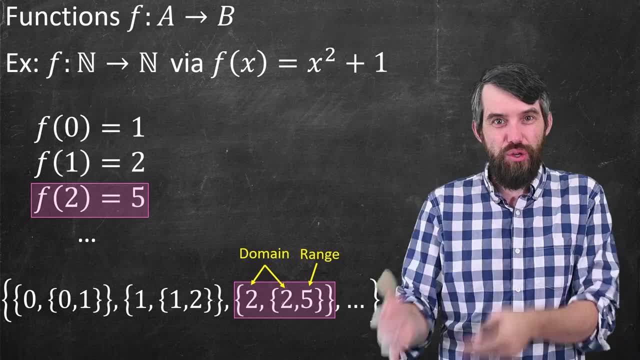 And then the squiggly bracket 2, 5 tells me that we're going to investigate setting 2, 2, 5.. So I love this method of encoding a function using set theory. This is just a set. It contains numbers, but we saw previously those themselves were just sets. 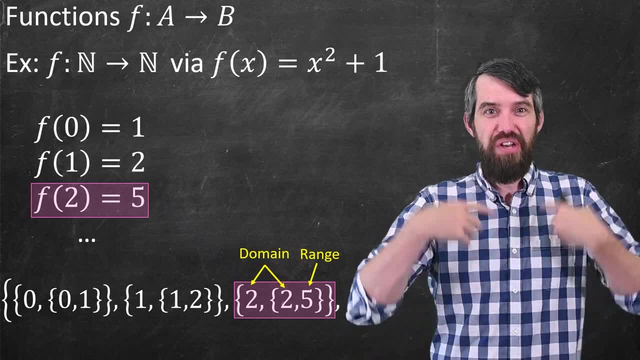 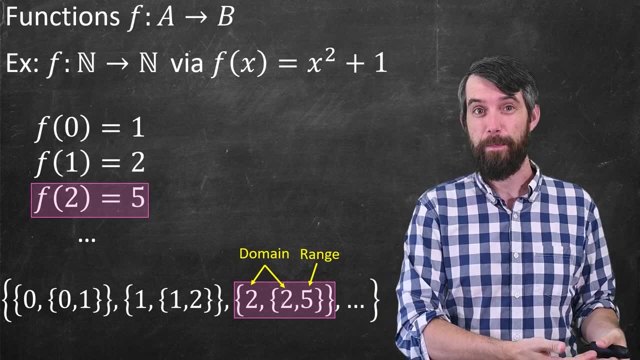 But put all of this together and now we have a notion of a function entirely in terms of a set, And I could write down some set in this way and you could tell me what the function was. Okay, so now I can actually state my definition of a function. 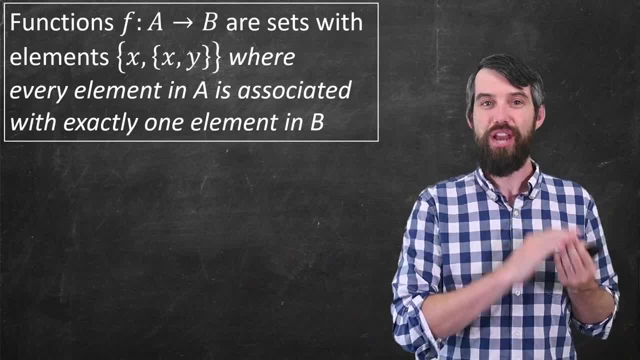 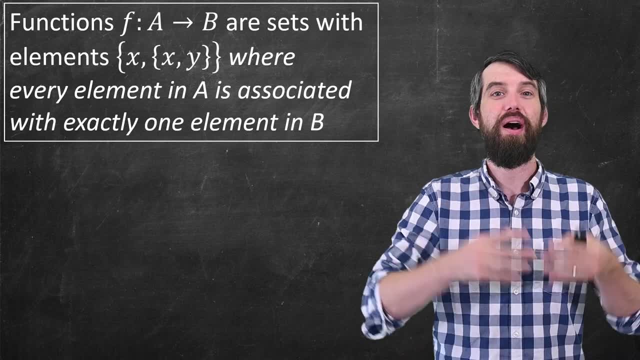 in terms of set theory, I'm going to say a function f from a to b Are sets whose elements look like what we just talked about: A squiggly bracket, x and then comma, a new set, xy- And I interpret this- where x are elements of a and y are elements of b. 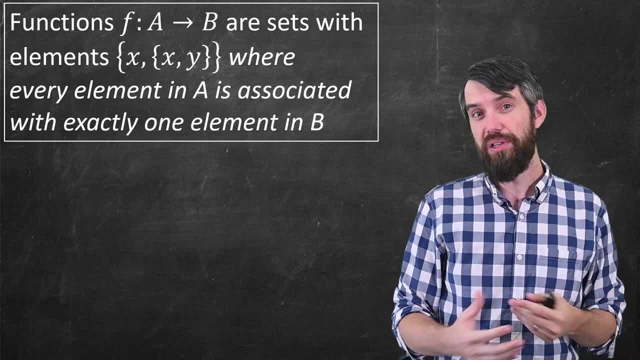 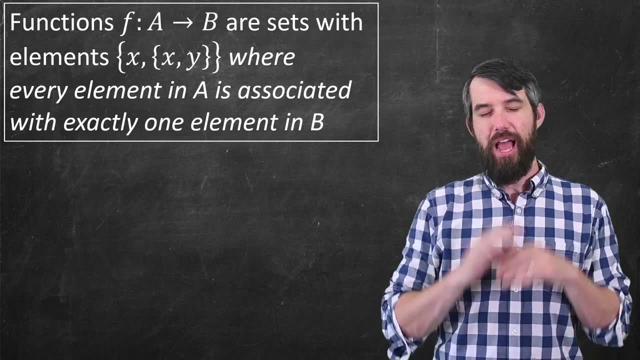 I do want to note, however, functions are not all things that look like this. You might have heard of, for example, the vertical line test for functions. Functions are sort of a special case And they must have this property that everything in the domain a. 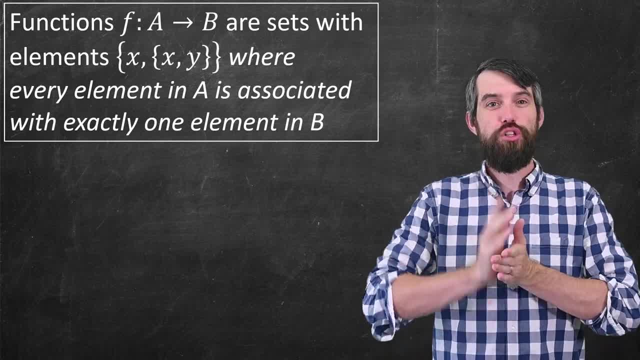 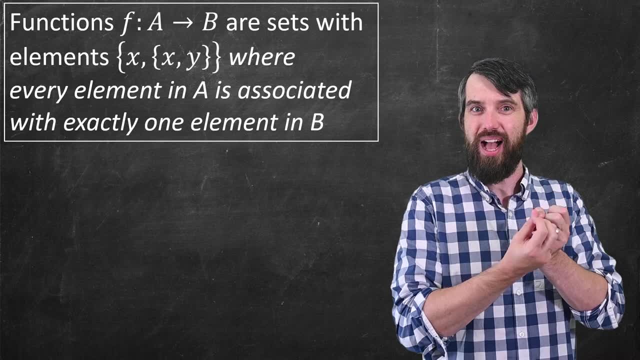 every element x in the domain a must be sent to exactly one other place. A function doesn't really make sense if you have one thing and you say what is f and the result is a couple of different values. So the function needs to take in all possible values from a. 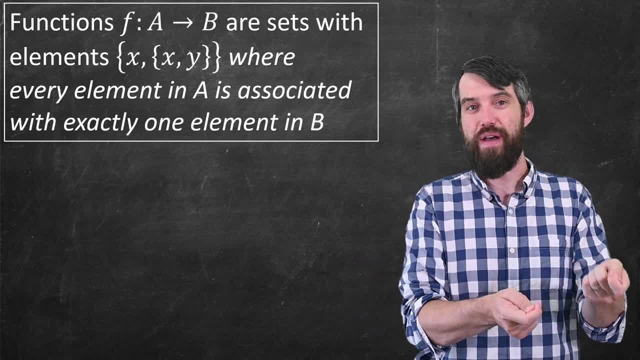 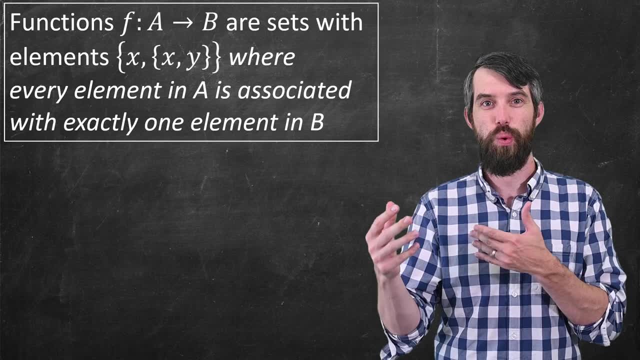 and only go for each individual value to exactly one value in b. So as long as the set that you've written down obeys these properties, then it represents a function and you can figure out what that function was. Now in practice. we don't actually really do this very often.